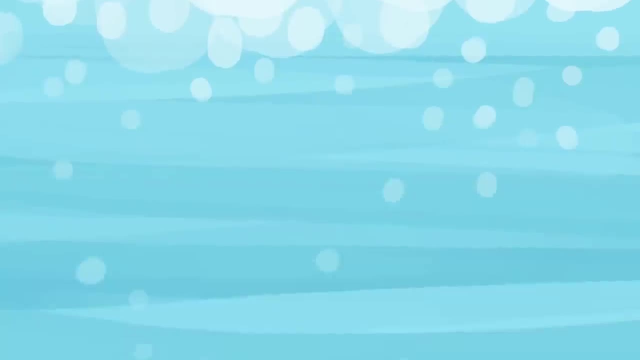 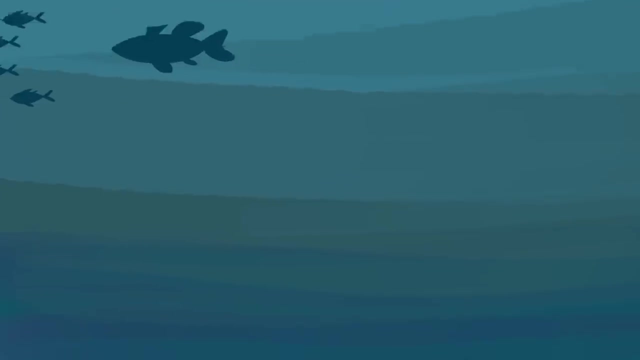 All of these technologies have enabled us to catch fish at greater depths and farther out at sea than ever before, And as the distance and depth of fishing have expanded, so has the variety of species we target, For example the Patagonian toothfish. 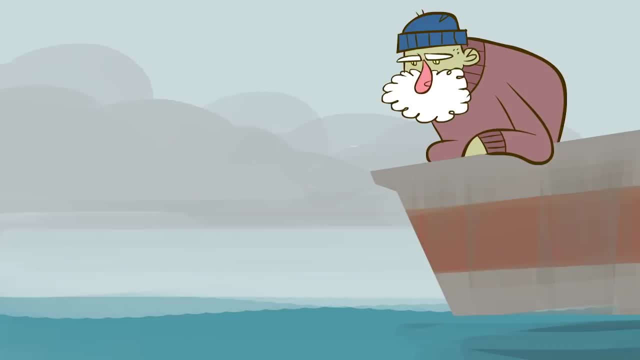 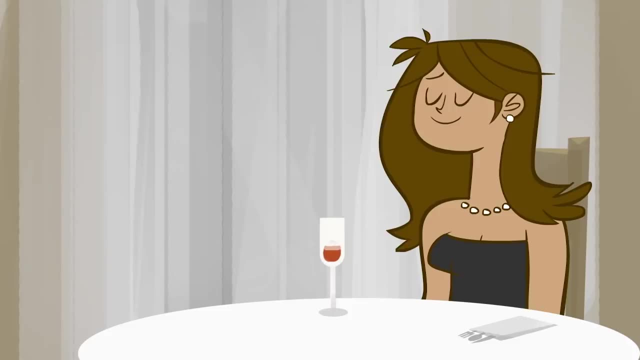 neither sounds nor looks very appetizing, and fishermen ignored it until the late 1970s. Then it was rebranded and marketed to chefs in the US as Chilean sea bass, despite the animal actually being a type of cod. 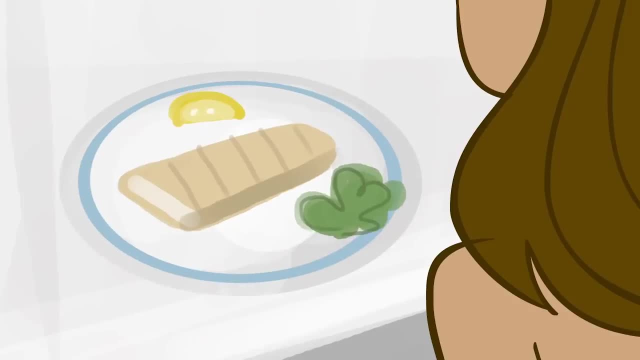 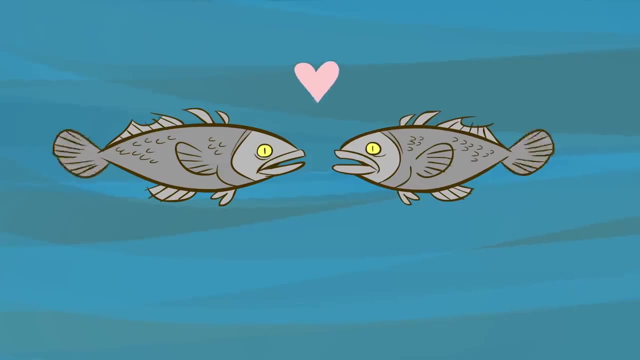 Soon, it was popping up in markets all over the world and is now a delicacy. Unfortunately, these deepwater fish don't reproduce until they're at least 10 years old, making them extremely vulnerable to overfishing when the young are caught before they've had a chance to spawn. Consumer tastes and prices can also have harmful effects. For example, shark fin soup is considered such a delicacy in China and Vietnam that the fin has become the most profitable part of the shark. This leads many fishermen to fill their boats with fins, leaving millions of dead sharks behind. 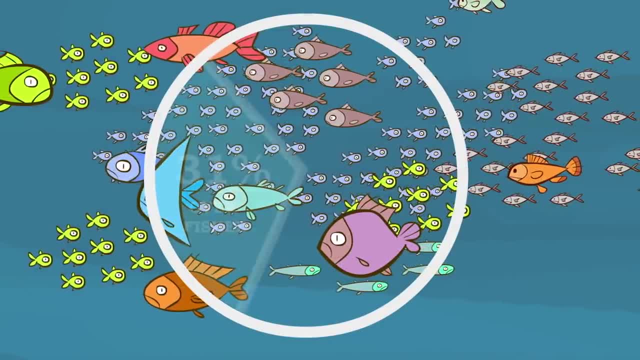 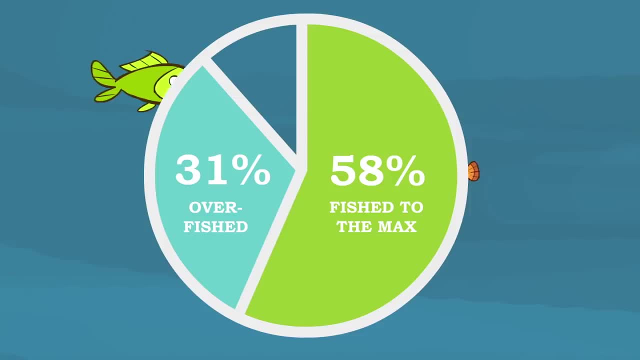 The problems aren't unique to toothfish and sharks. Almost 31% of the world's fish populations are overfished and another 58% are fished at the maximum sustainable level. Wild fish simply can't reproduce as fast as 7 billion people can eat them. 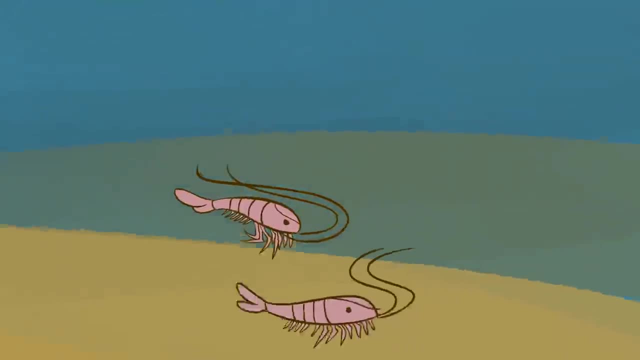 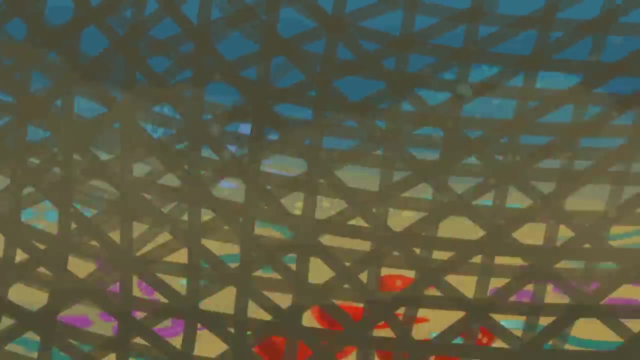 Fishing also has impacts on broader ecosystems. Wild shrimp are typically caught by dragging nets the size of a football field along the ocean bottom, disrupting or destroying seafloor habitats. The catch is often as little as 5% shrimp. The rest is bycatch. 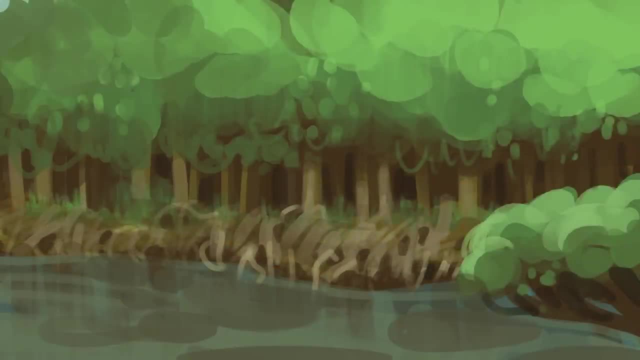 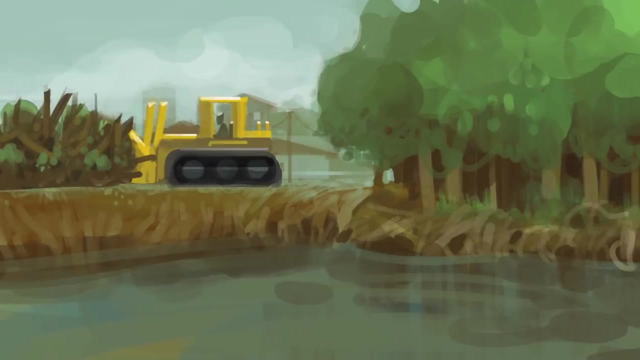 unwanted animals that are thrown back dead, And coastal shrimp farming isn't much better. Mangroves are bulldozed to make room for shrimp farms, robbing coastal communities of storm protection and natural water filtration, and depriving fish of key nursery habitats. 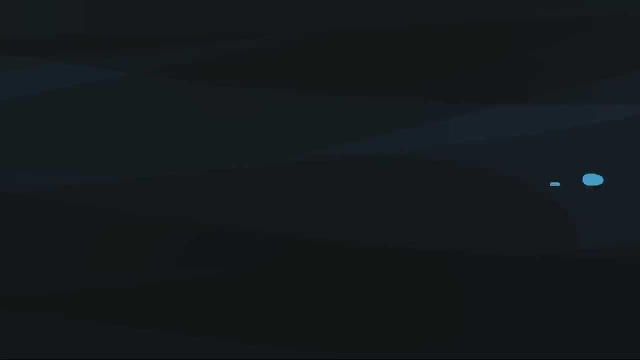 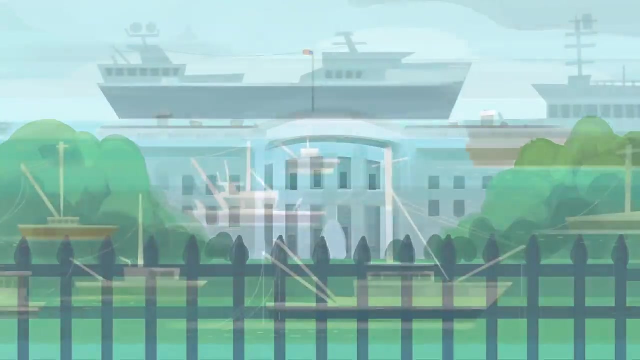 So what does it look like to give fish a break and let them recover? Protection can take many forms. In national waters, governments can set limits about how, when, where and how much fishing occurs, with restrictions on certain boats and equipment. 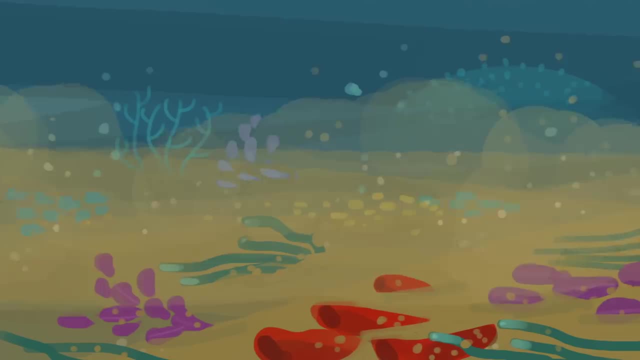 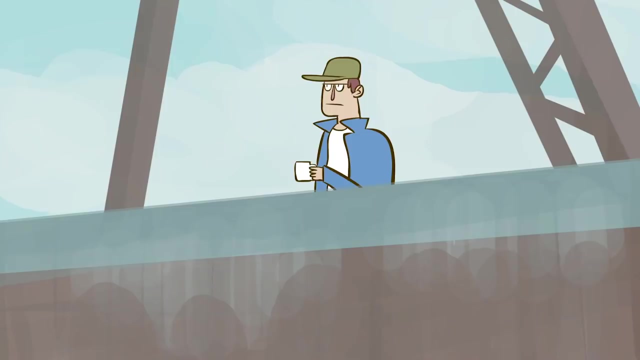 Harmful practices such as bottom trawling can be banned altogether and we can establish marine reserves closed to all fishing to help ecosystems restore themselves. There's also a role for consumer awareness and boycotts to reduce wasteful practices like shark finning.